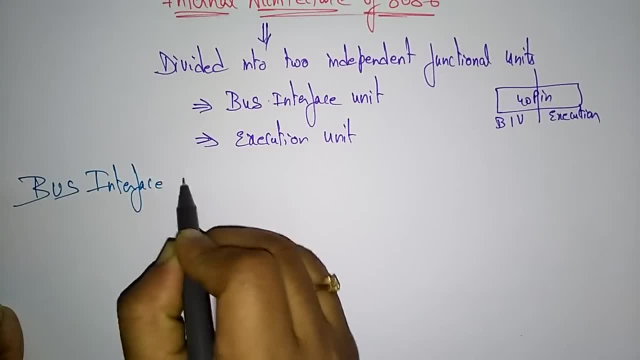 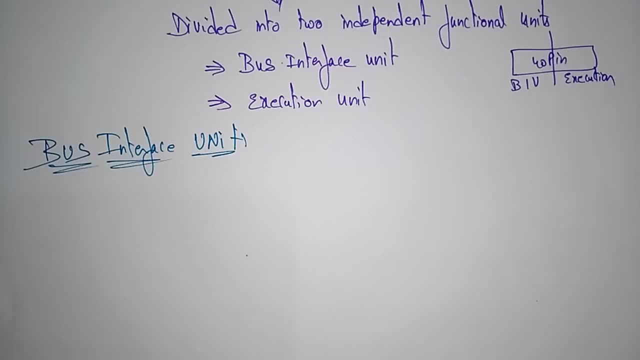 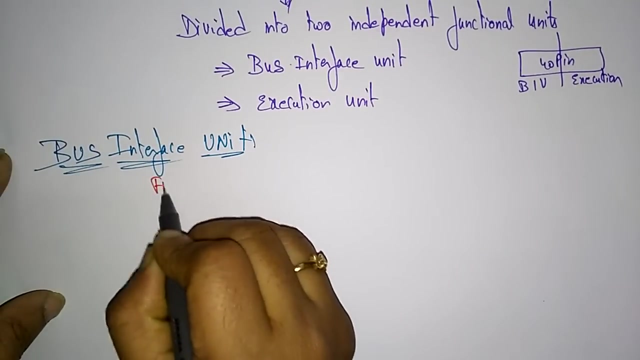 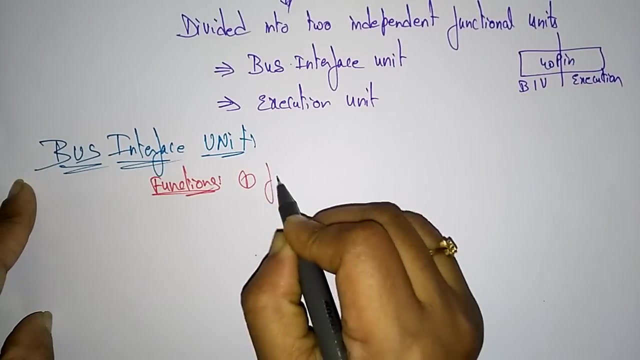 Bus interface unit. So first let me explain about the bus interface unit. So what is the use of the bus interface unit, What it does, What are the functions that this bus interface unit is having? Let us see the functions. So the first, the bus interface unit: fetch the instruction means taking the instructions. 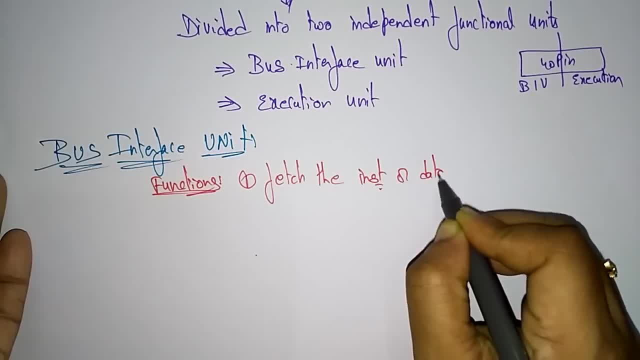 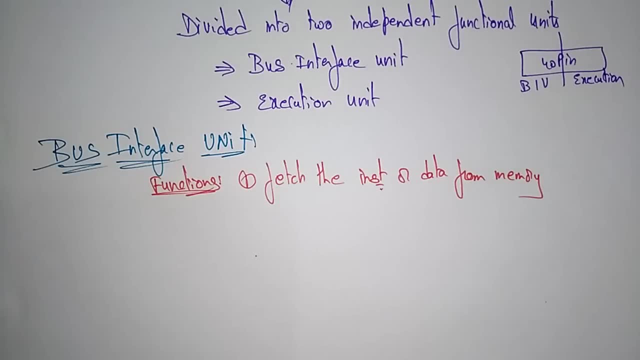 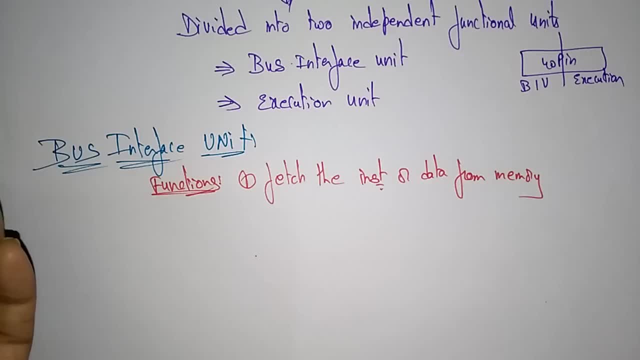 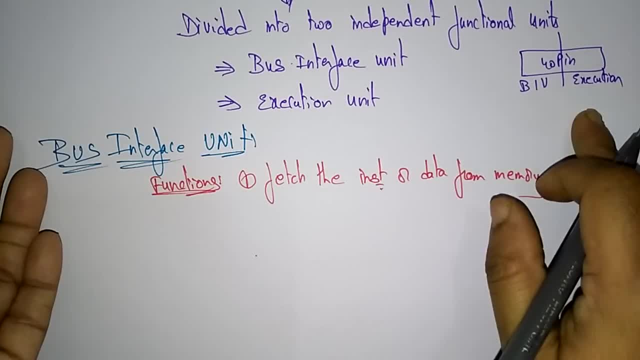 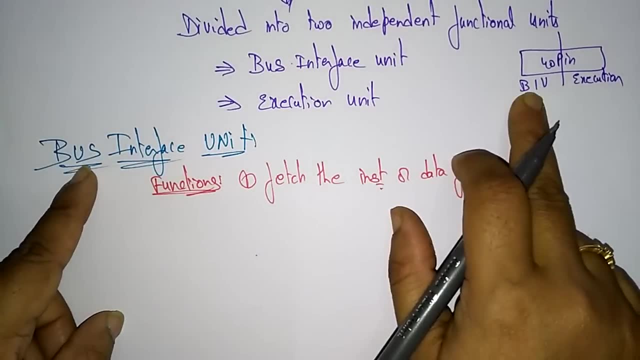 So the execution unit wants to execute some data, So what data it has to execute? That data will be fetched by the bus interface unit. So the first function of bus interface unit is to fetch the instruction or data from memory. Okay, 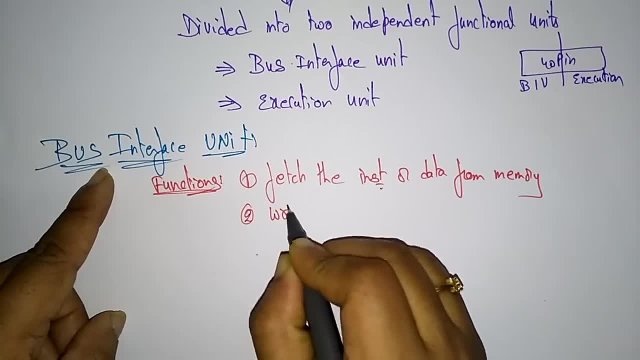 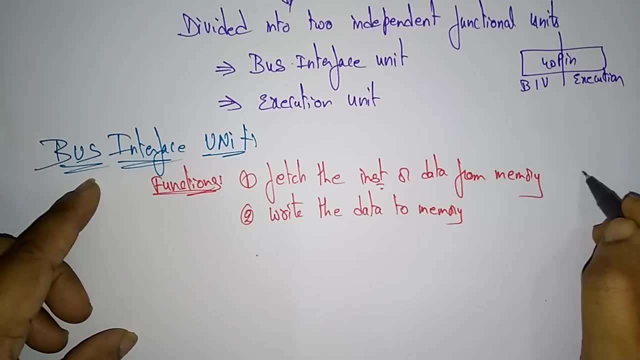 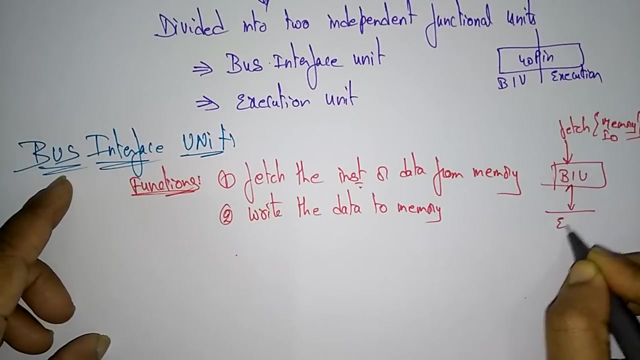 it fetch the data, so next it write the data to memory. okay, it's also doing another work, like, so it is fetching the data from where? from memory or IO. so this bus interface unit is fetching the data execution and so so this completely in the processor. the processor is divided into bus interface. 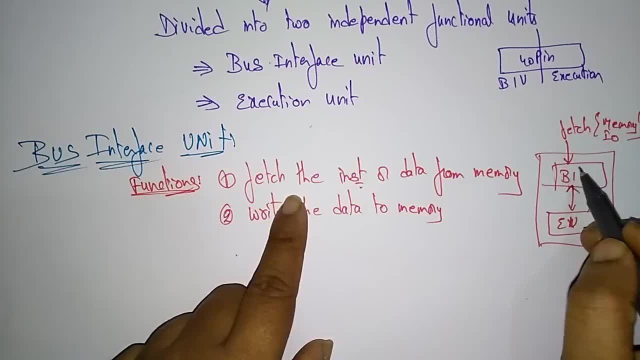 unit and the execution unit. so first the pro bus interference: fetch the deh physician, the unit fetch the data from memory and I O and send that data to the execution unit. so after that it performs some operation, the execution unit will perform some operation and send the data to the bus interference. then what this? 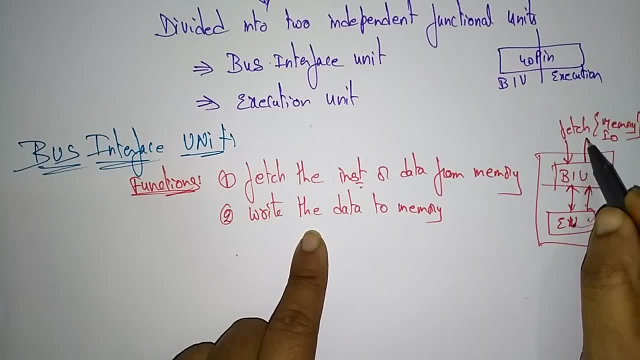 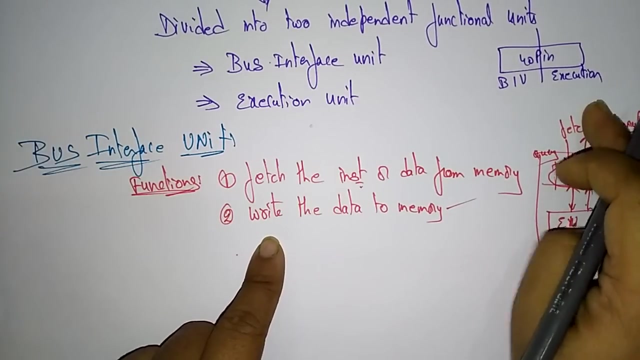 bus interface unit will do it write the data to means. this is a result. this is a query. okay, so after performing the operation, the execution unit will send that information to bus interface unit. then the role of the bus interface unit is to write the data to memory. it fetch the data at the same time. it write the data to. 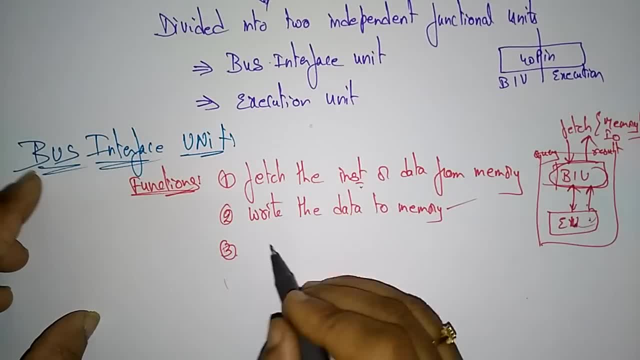 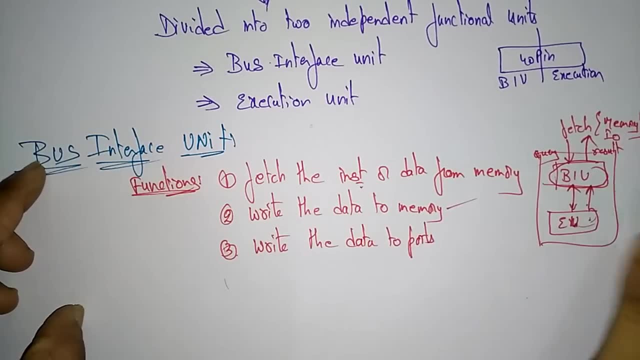 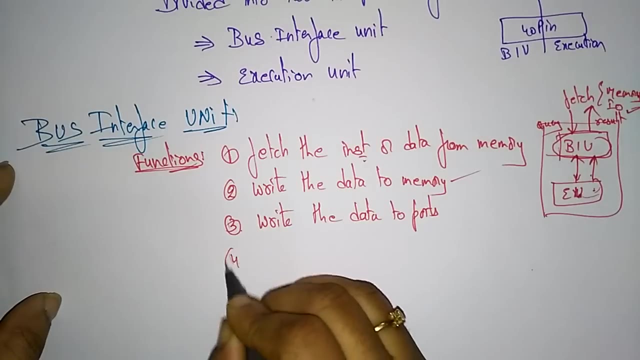 memory. okay, and next, and it also write the data to ports also. so ports is nothing but input output ports. so it is sending the data to memory as well as to the input output ports and also it does the work as it reads data from ports. 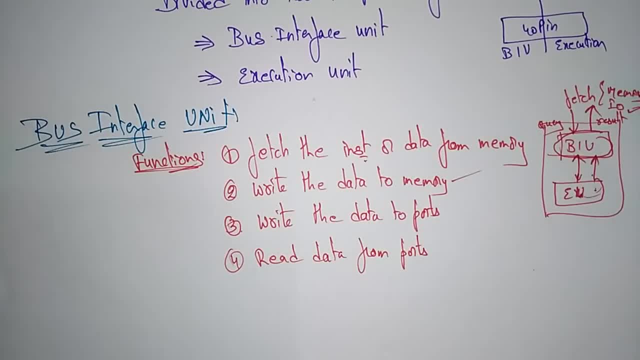 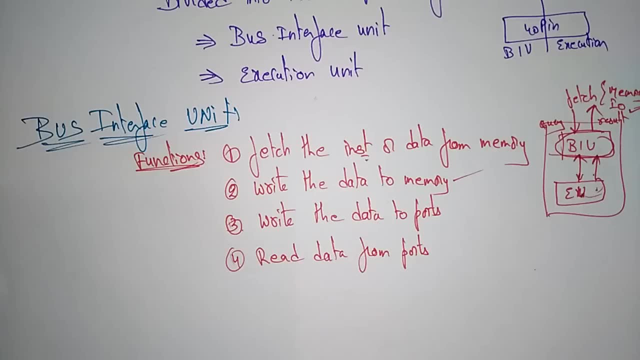 so this is a simple information. the bus interface unit is always taking and giving. that's it. so from where it is taking, it's fetching the data from memory. after that it write the data to memory and also it write the data to input output ports and also it read. 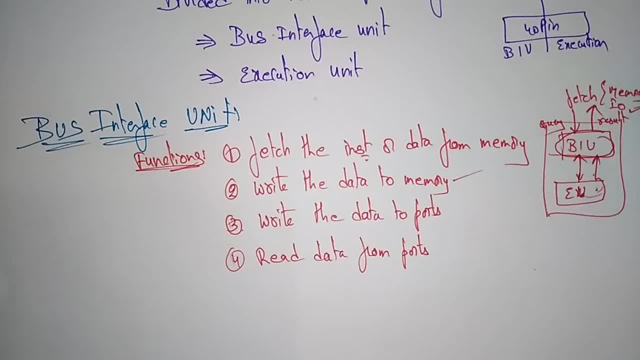 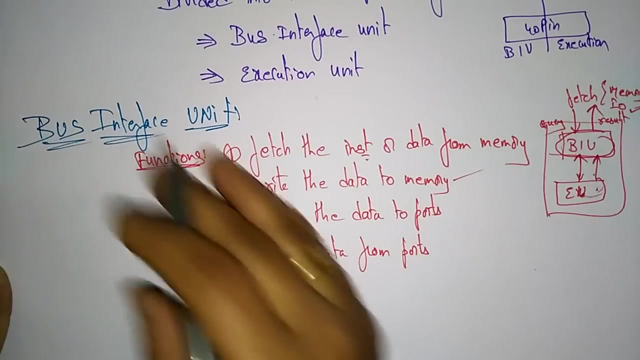 the data from ports means fetch the data from ports, fetch the data from ports and memory and write the data to ports and to memory. so that is the work of the bus interface unit. so the bus interface unit consist of three functional parts. so this unit is divided. 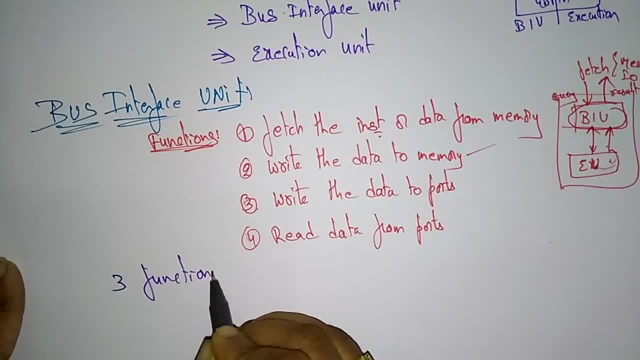 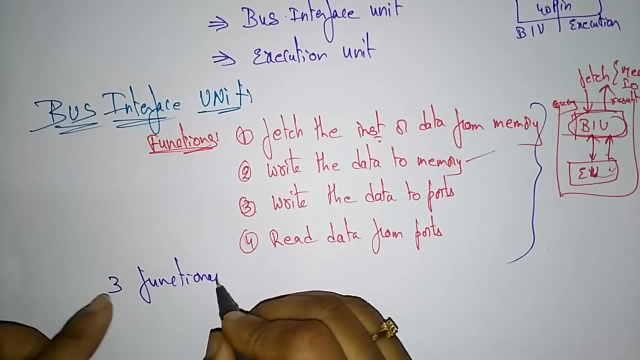 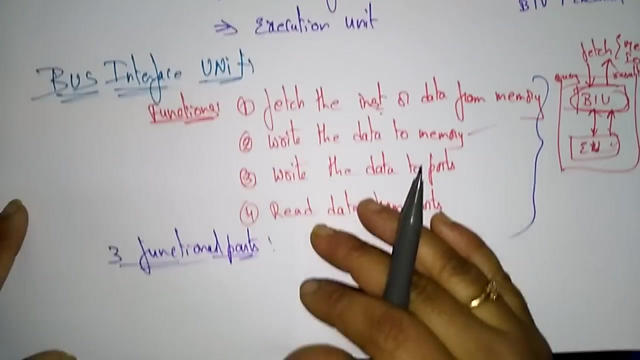 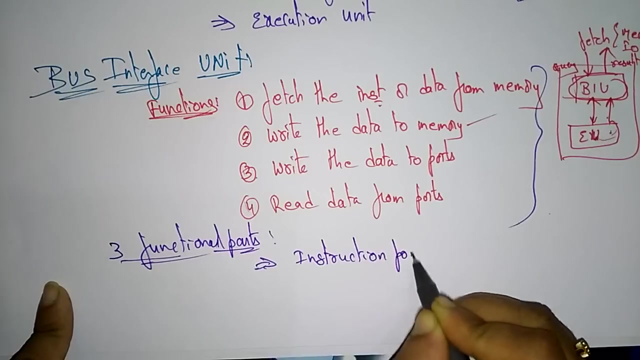 into three functional parts. We had seen the functions, so which devices is doing this functions in the bus interface unit. that is this, the functional parts. so this three functional parts will do this. four works. those are instruction pointer, instruction pointer, IP and segment register. 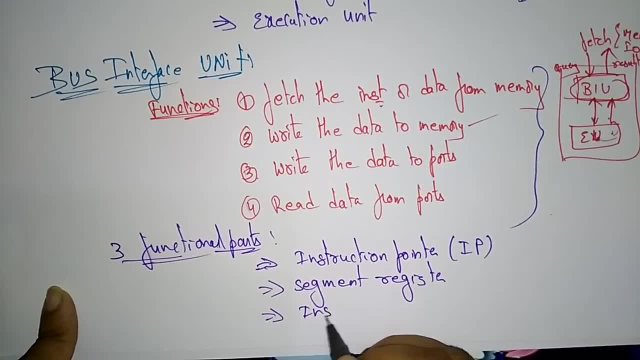 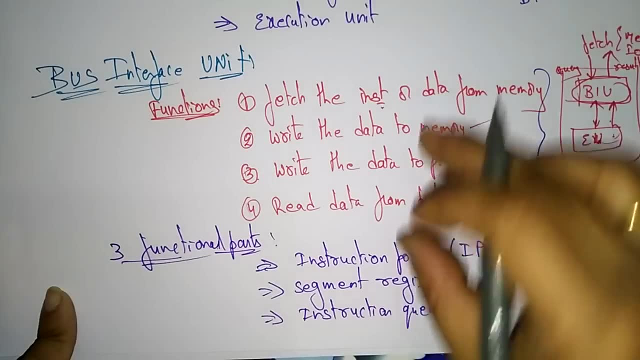 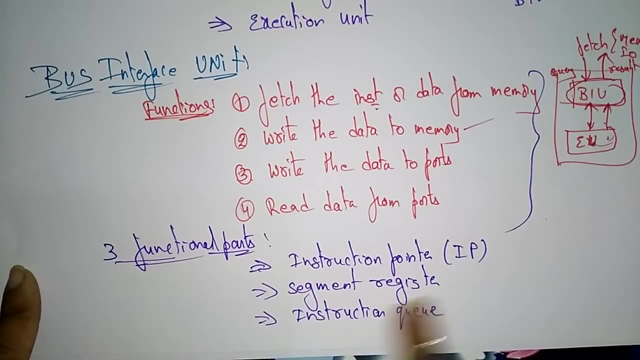 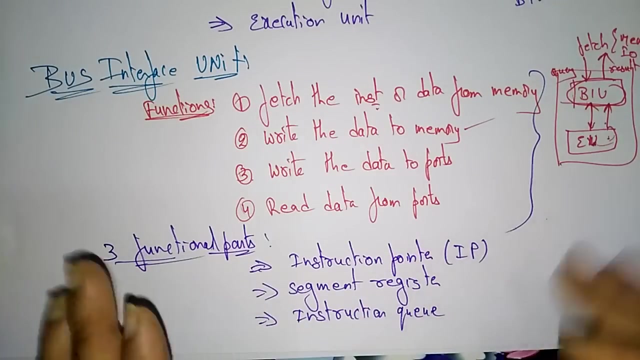 next instruction queue. so these are the three functional units which perform these operations. means these operations will be divided in three functional units: instruction pointer, segment, register, instruction queue. first let me explain about these functional parts. after that I will show you this operation in the diagram. okay, so let explain the. 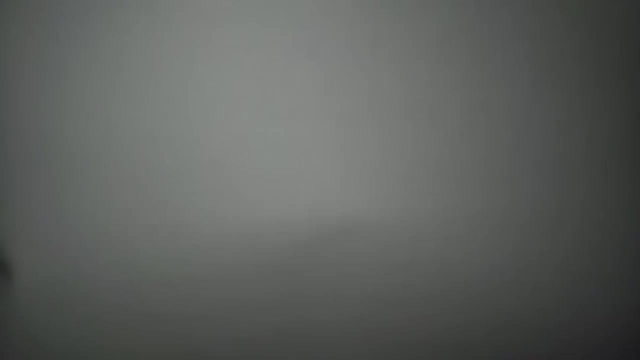 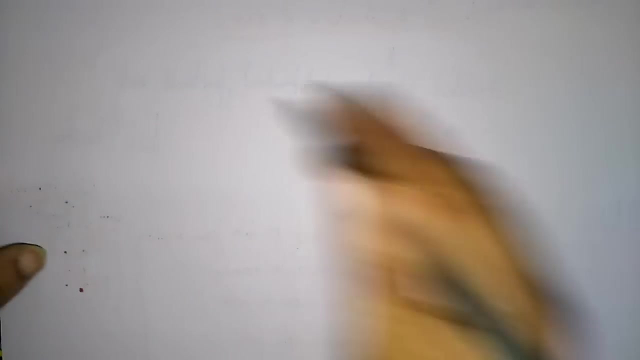 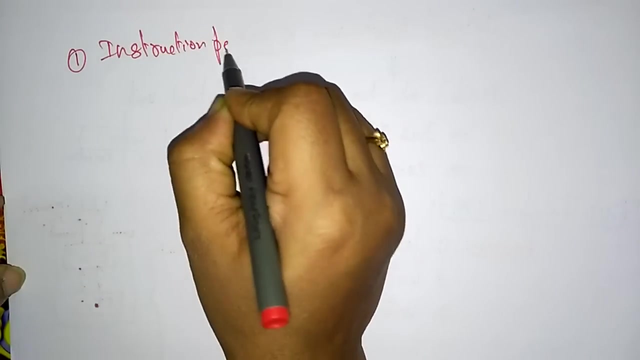 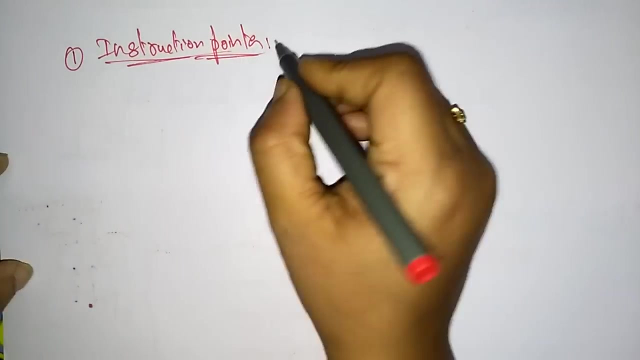 instruction pointer. so what is the use of instruction pointer in the bus interface unit? so the first functional part is instruction pointer. so what is the role of instruction pointer? so the instruction pointer first? it is a sixteen bit, it is a sixteen bit region. 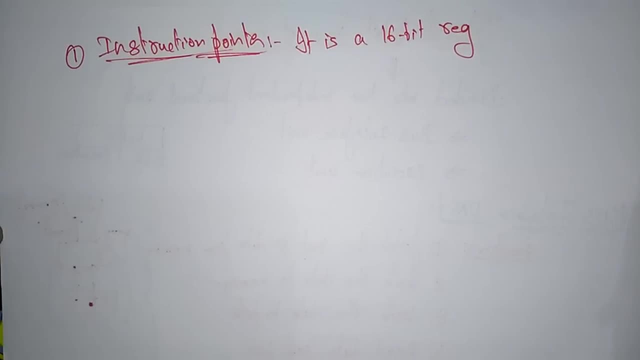 okay, So instruction pointer itself is a register. everything the data is stored and send, everything will be done with the help of only registers. so you have to talk about the registers whenever you are sending the data and retrieving the data and doing the operations everything. 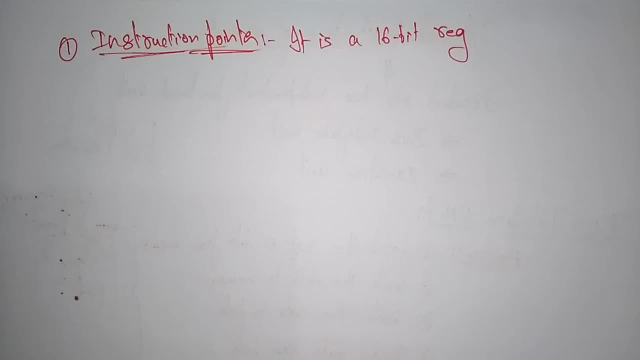 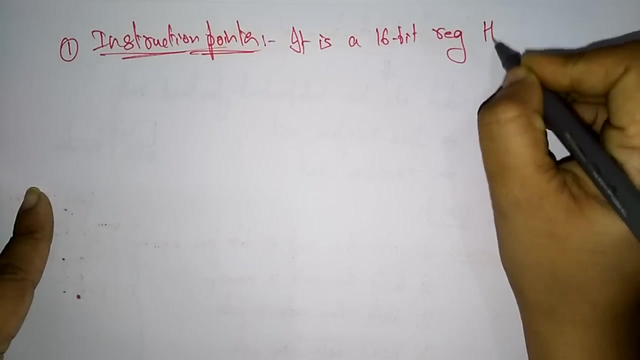 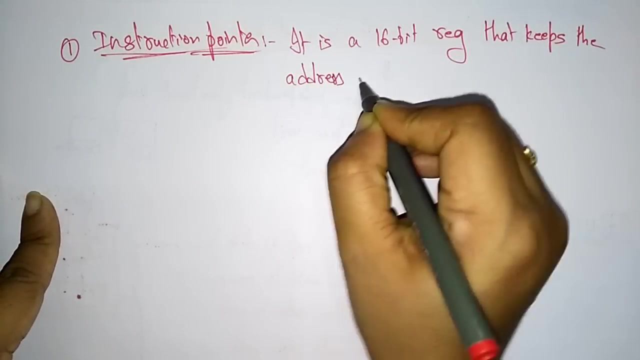 will be based on the registers. okay, so in the registers you are having the data in the form of bits. do not be confused. registers holds the data. that data is everything in the form of bits. So instruction pointer is a sixteen bit register that keeps the address. address of 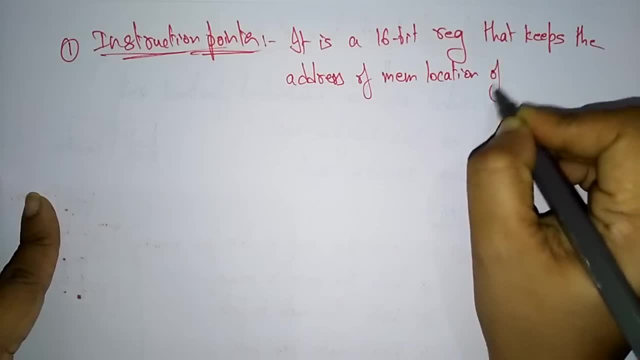 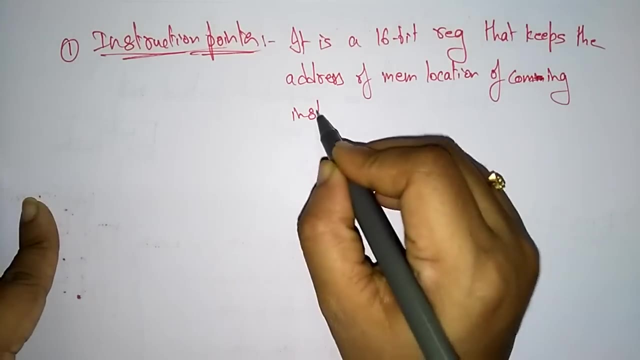 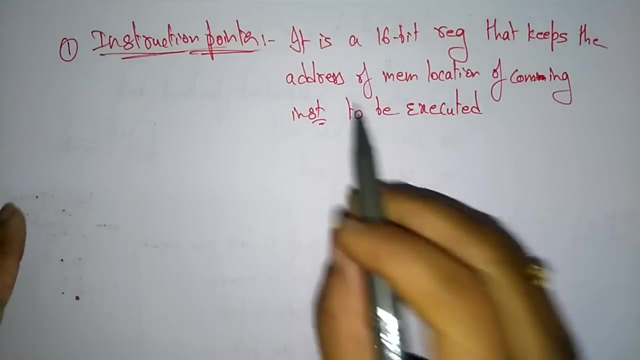 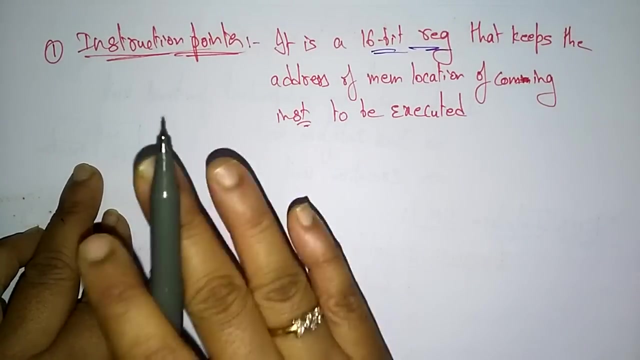 memory location of coming instruction to be executed. coming coming instruction to be executed. that is the role of this instruction pointer. Okay, Yes, So instruction pointer first. it is a sixteen bit register. what is the operation that is this instruction pointer will do? 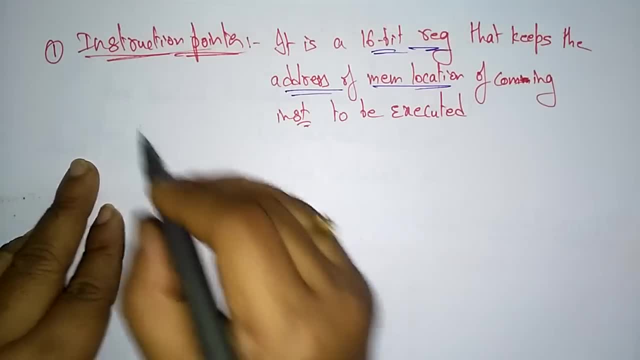 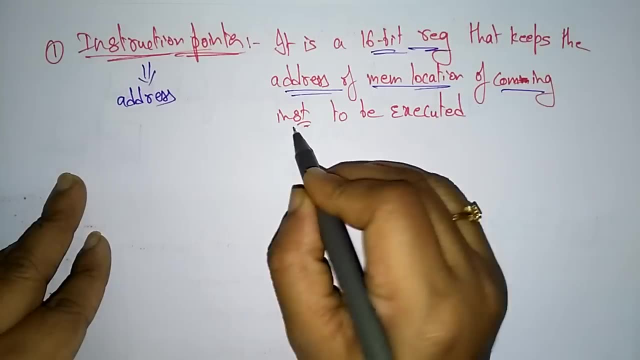 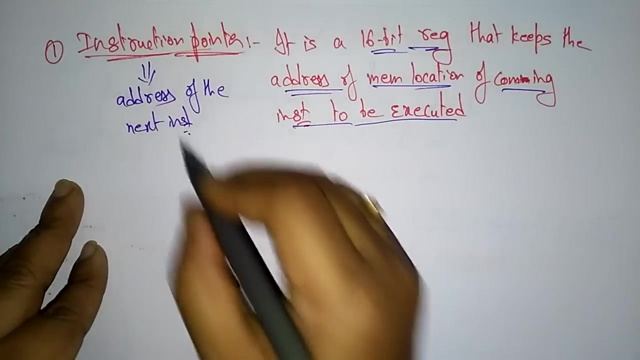 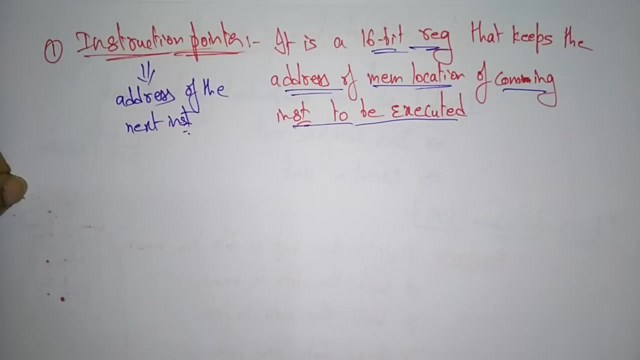 This register will keep the address of memory location only. it holds the address. address of memory location of coming instruction to be executed, address of the next instruction, next instruction to be executed. so this instruction pointer holds the address of the next instruction to be executed. So that is the instruction pointer. Next is the segment register. So 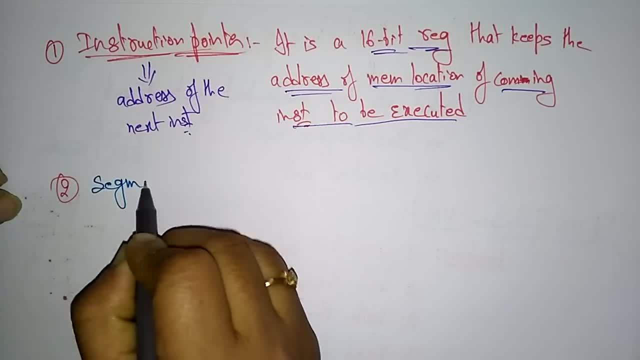 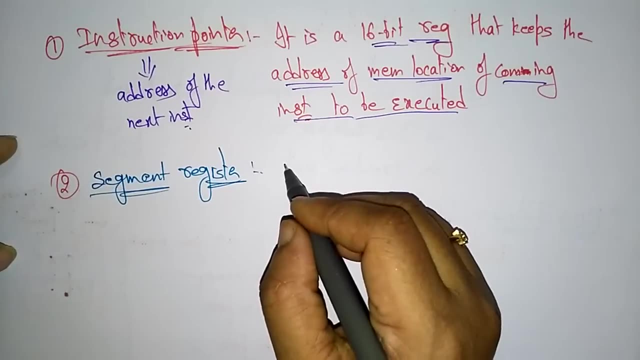 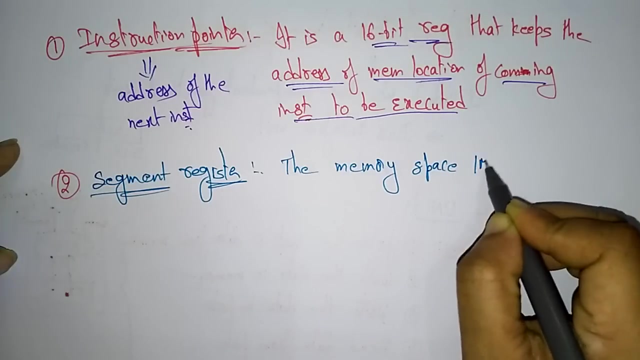 second one is the segment registers that are present in the bus interface unit. So what is the role of the segment register Here? the memory space: the memory space that is 1 megabyte. I already said in the features that 8086 is having the addressing capacity. 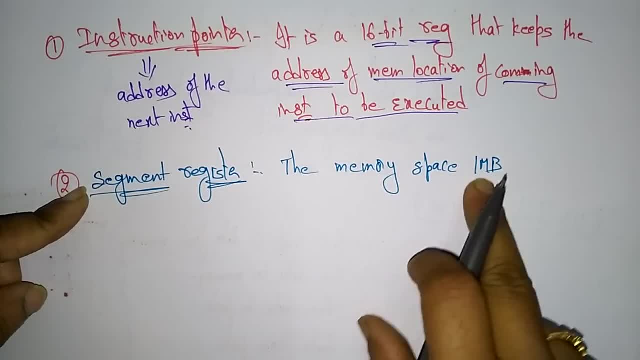 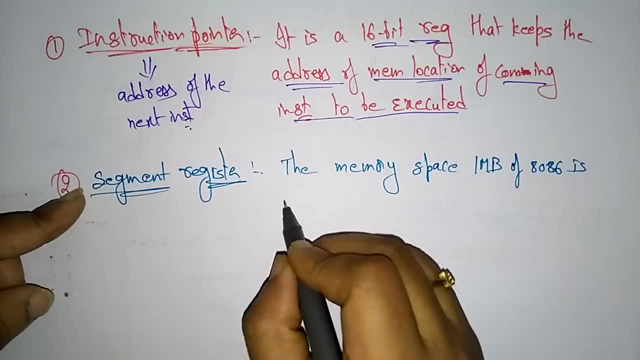 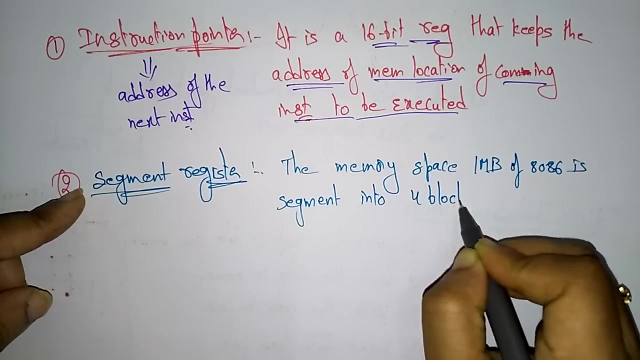 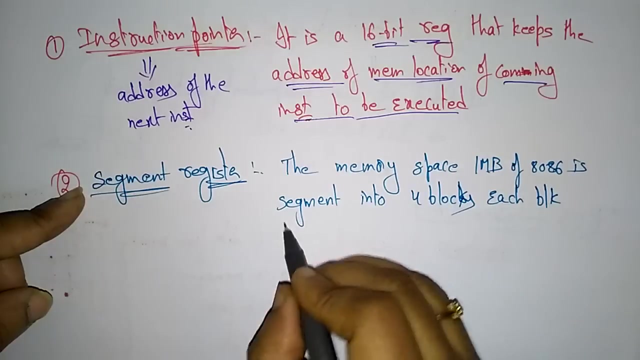 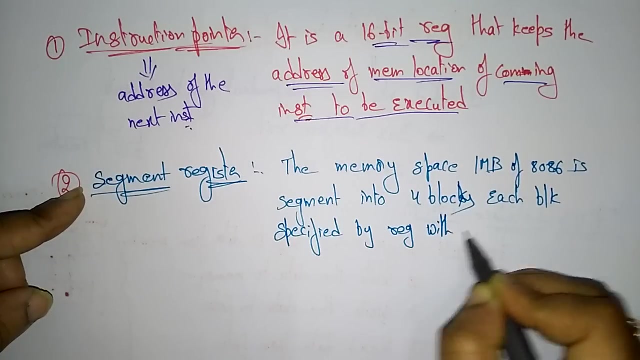 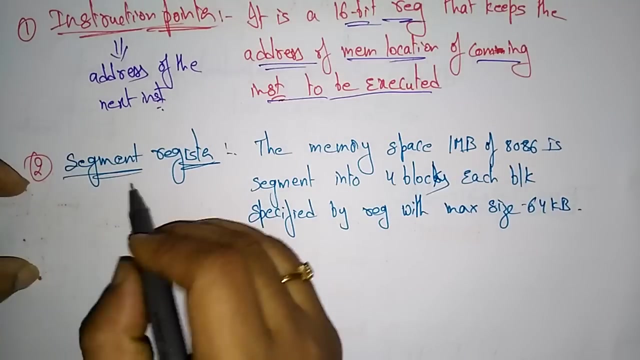 as 1 megabyte. So this segment register holds 1 megabyte of memory of 8086 is. segmented means divided. segmented means divided, divided into 4 blocks, 4 blocks. Each block specifies by register with the maximum size: 64 bit. 64 kilobyte means the complete segment registers. 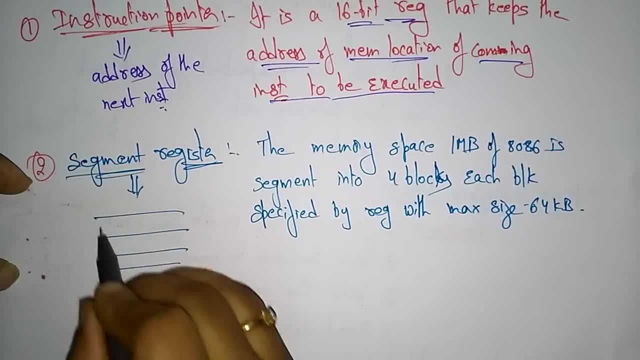 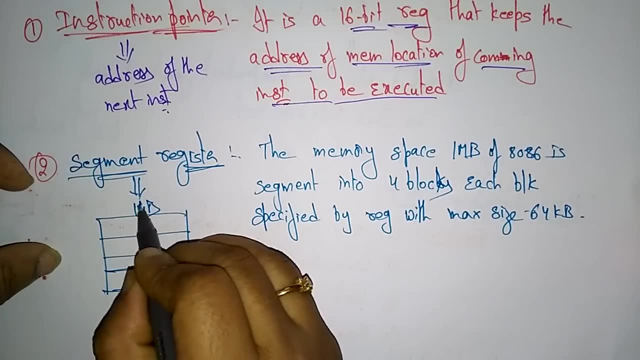 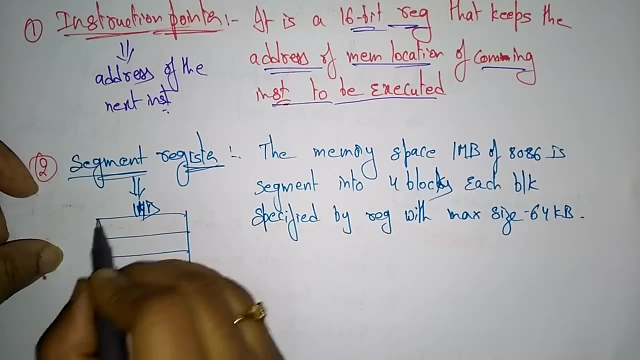 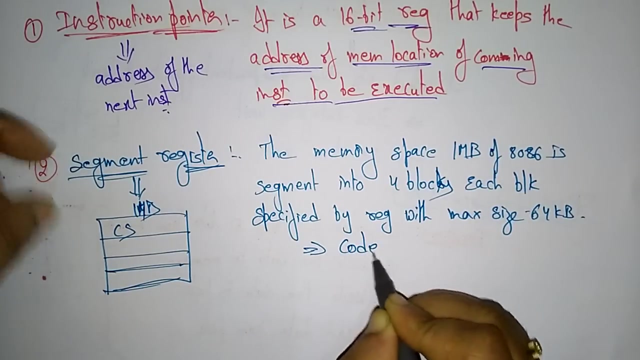 is divided into 4 blocks. This is completely 1 megabyte, So 1 megabyte register. So here in each block specifies. So the 4 segments are the core segment. Let me write that The 4 registers that are used. 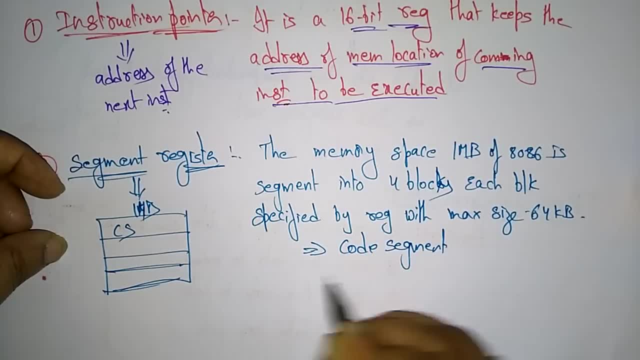 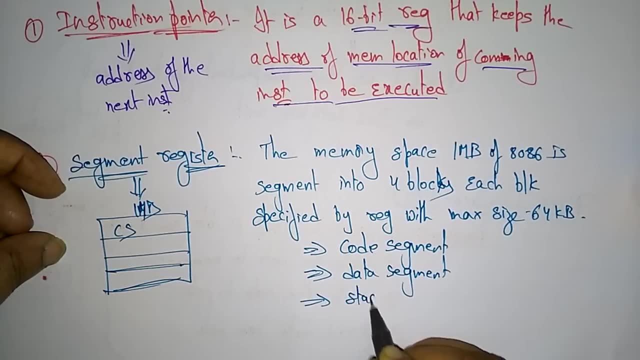 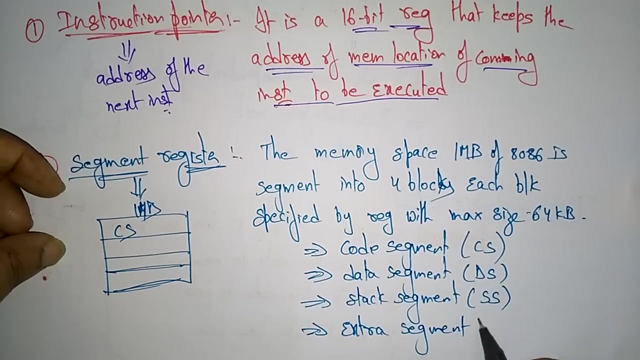 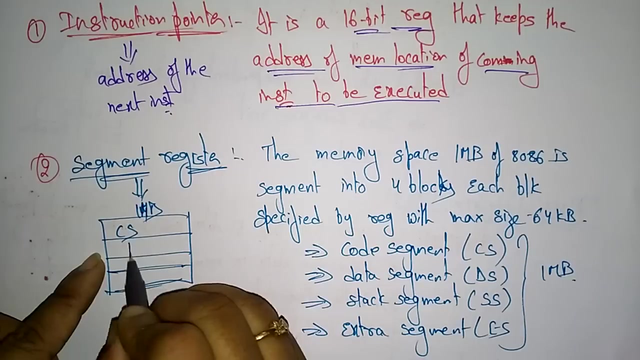 in the segment register are core segment, data segment, stack segment and extra segment, Extra segment. So this is a core segment, data segment, stack segment, extra segment. So this completely of 1 megabyte, But each segment: core segment, data segment, stack segment, extra segment. 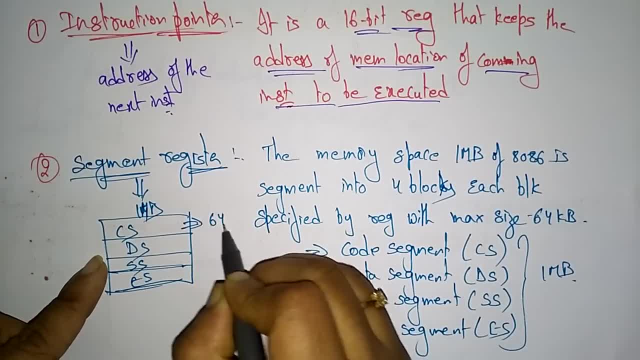 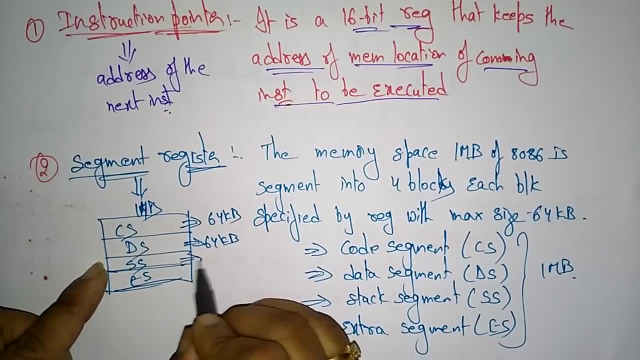 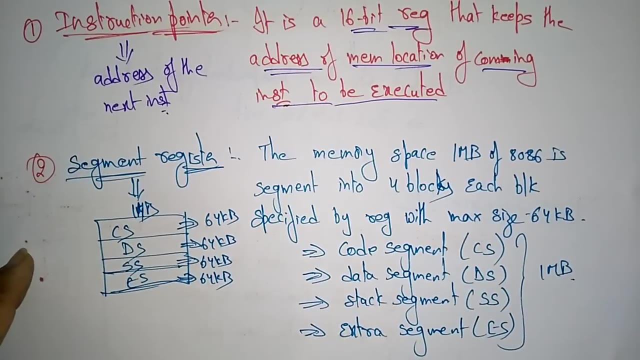 is divided into 4 blocks. Each block holds 64 kilobytes of memory Each register, so this you call it as a registers to store the data. So each can hold 64 kilobytes of data at a time, So up to 64 kilobytes it can store. So this is about the segment register. So the next. 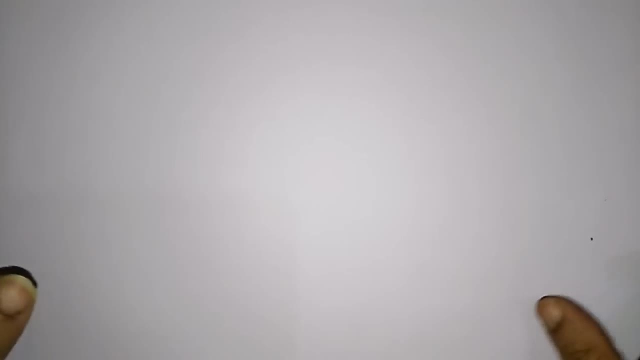 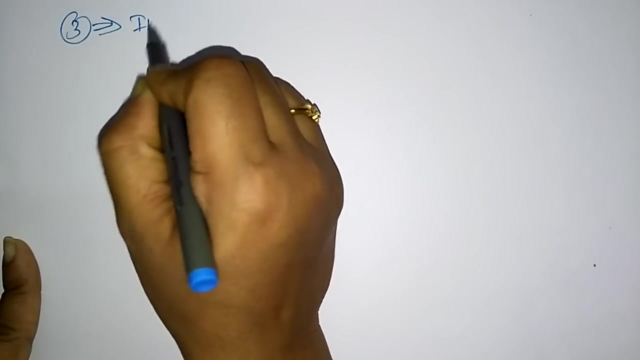 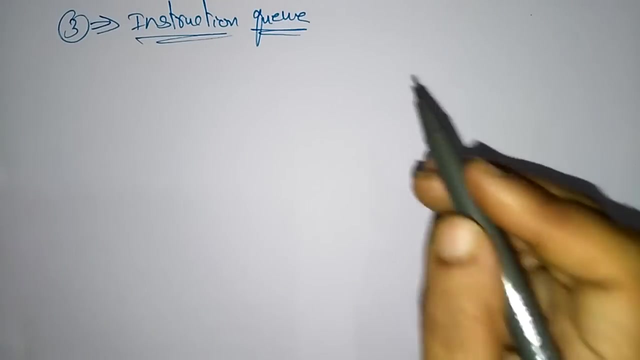 register is sorry. the next functional unit is. there is a third one. This is instruction queue. Instruction queue. So the bus interface unit is divided into 3 functional parts. So 1 is the instruction pointer which holds the data. So 1 is the instruction pointer which. 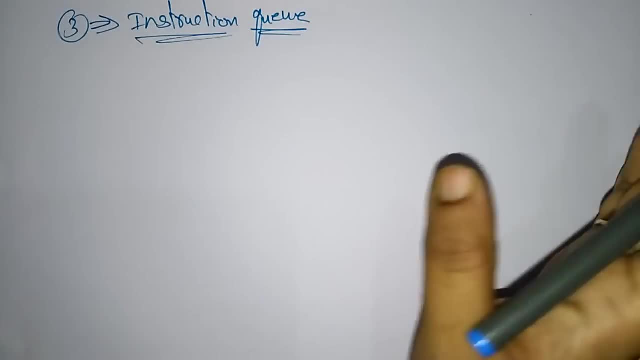 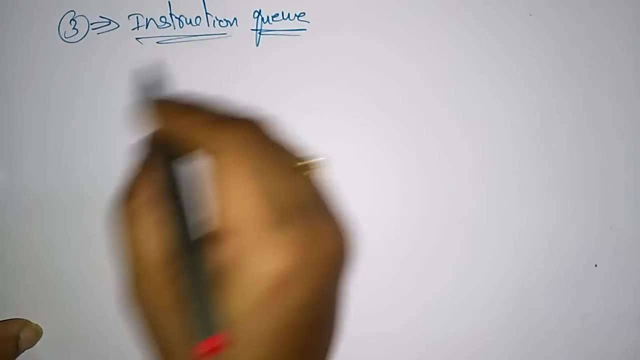 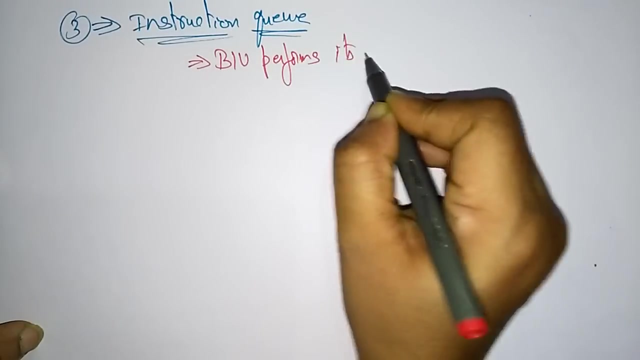 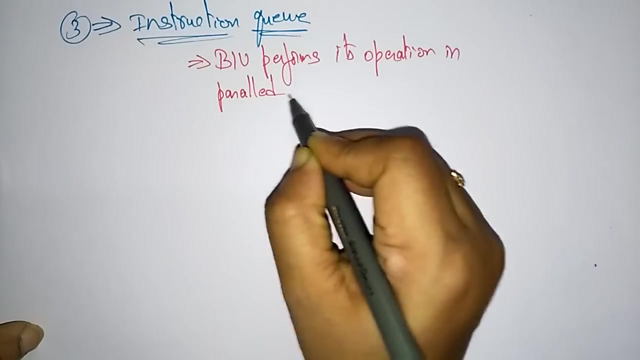 holds the address of the next 3 instructions Segment register is having the 4 segment uh to store the data. And next is the instruction queue. What is the role of the instruction queue? So here the bus interface unit performs, performs its operation in parallel with- sorry, parallel with execution To show the values. here it 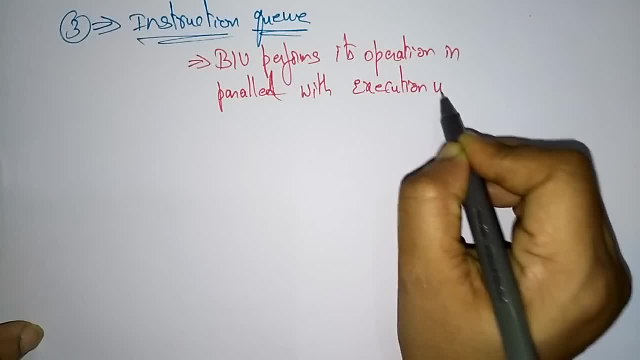 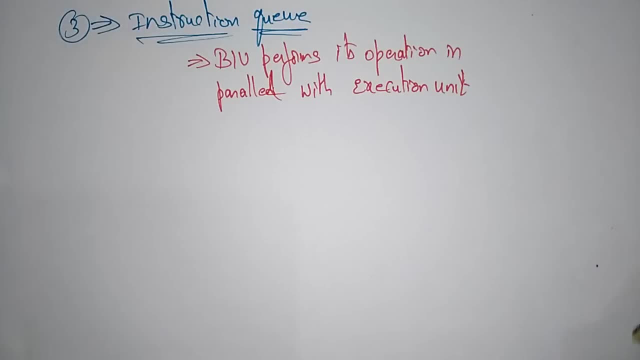 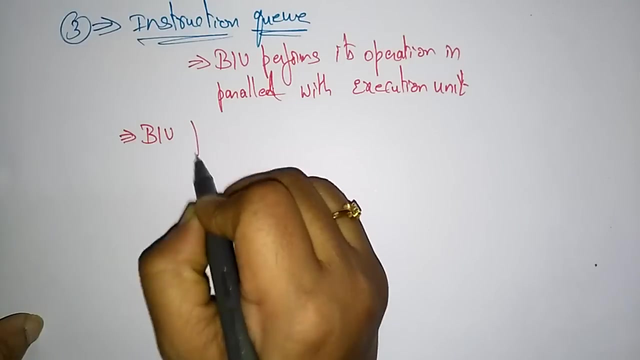 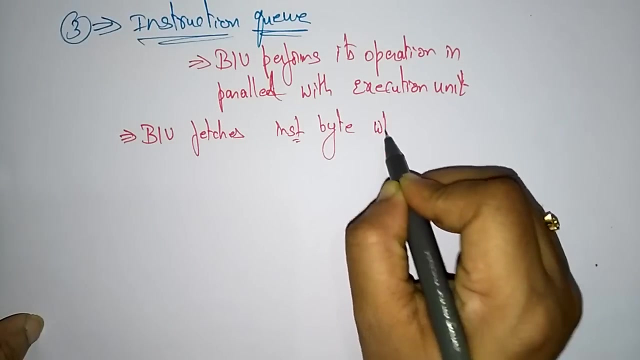 is구 unit. So the bus interface unit. it performs its operations. So whatever the operations it is performing, is parallel with execution unit. and here the bus interface unit fetches instruction byte first. it fetches instruction byte while execution, So in while execution. 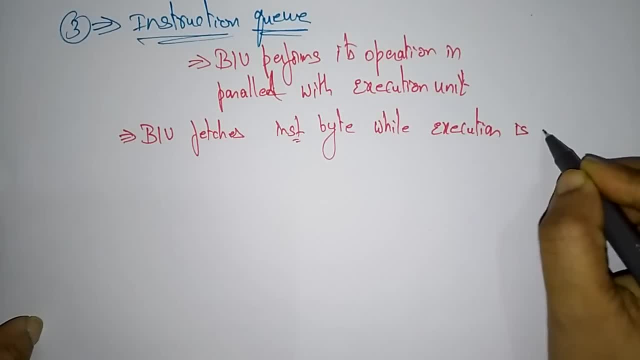 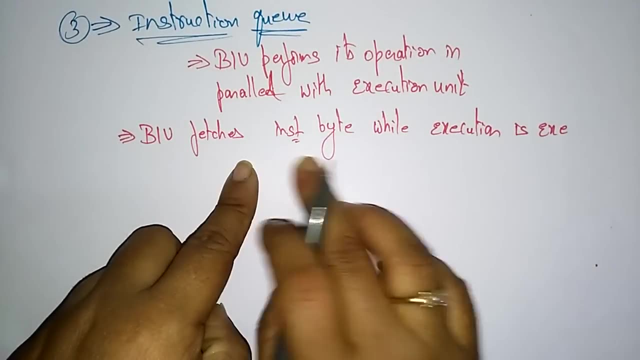 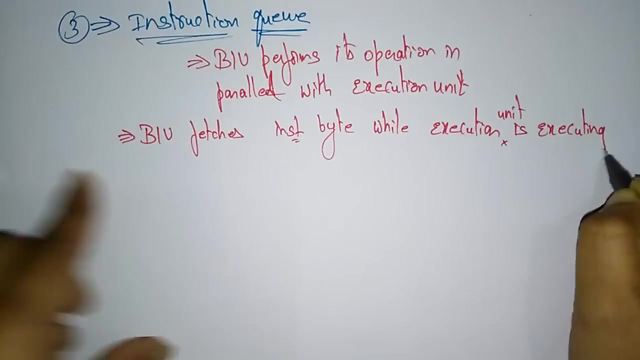 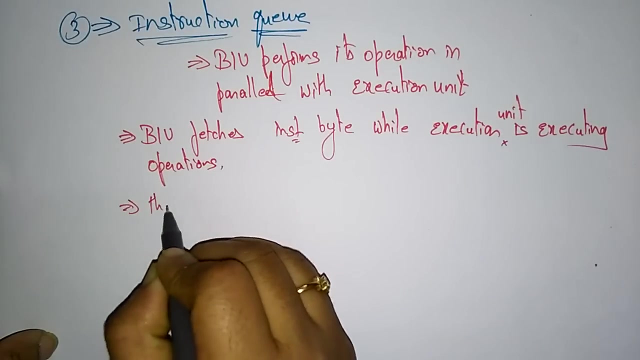 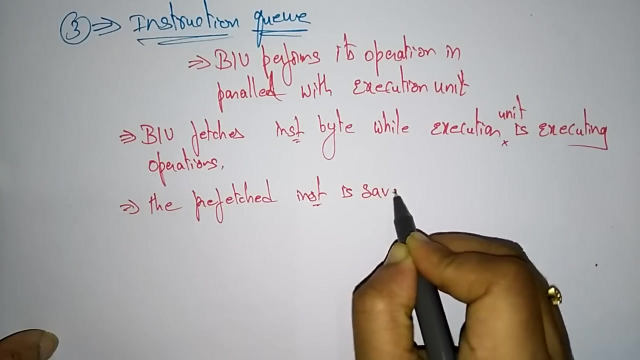 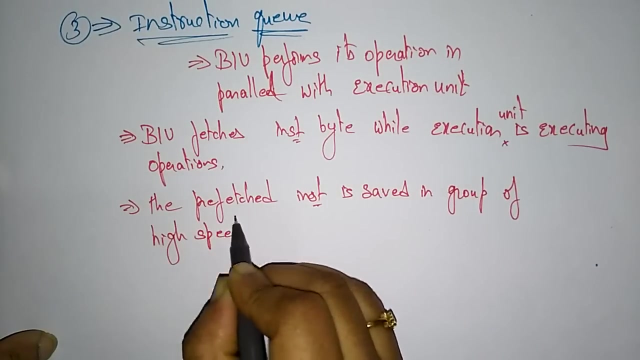 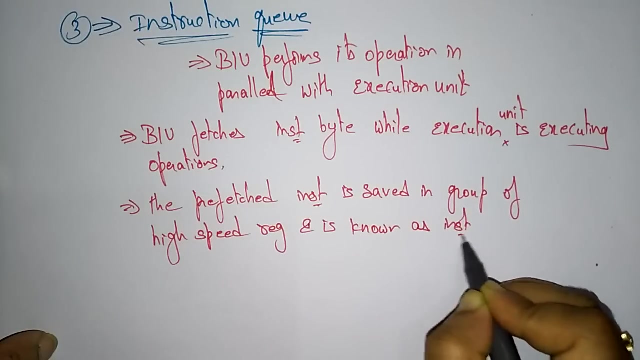 it fetches the instruction byte in is executing operations. sorry, execute bus. interface unit fetches instruction byte while execution unit is executing operations. Next, the prefetched bus. the prefetched instruction is saved in group of high speed registers and is known as instruction queue instruction. 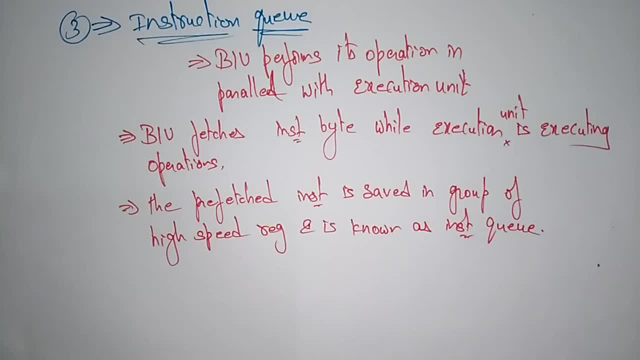 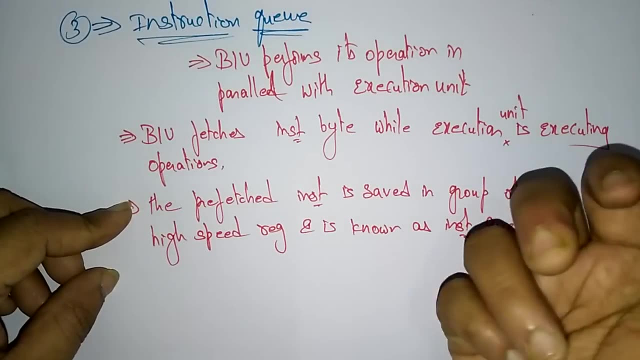 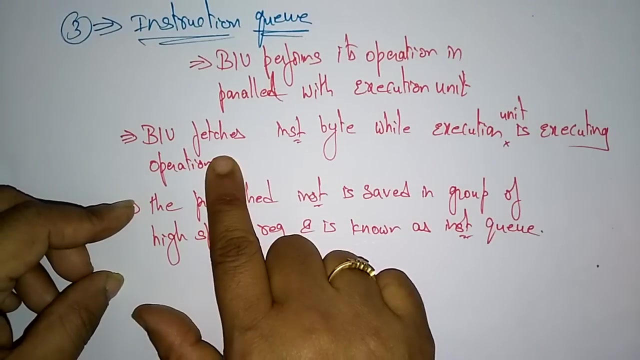 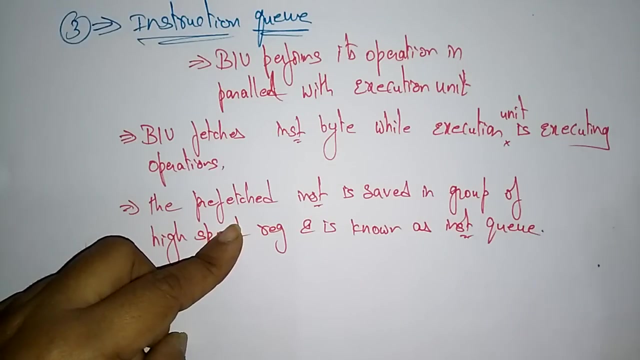 queue. So what this instruction queue will do? first, the bus interface unit fetches instruction byte while execution unit is executing operation. So whatever the execution unit is executed, the data immediately, so that the pre fetch instruction is saved in the high speed registers, is known. 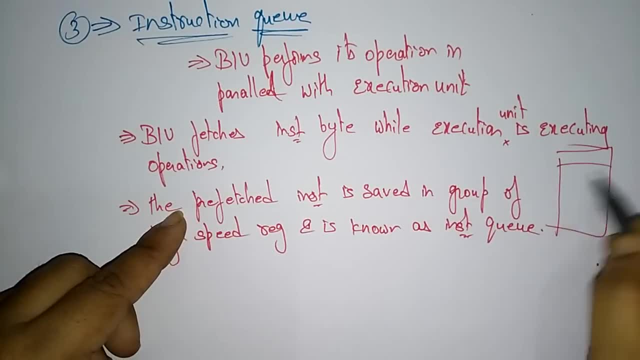 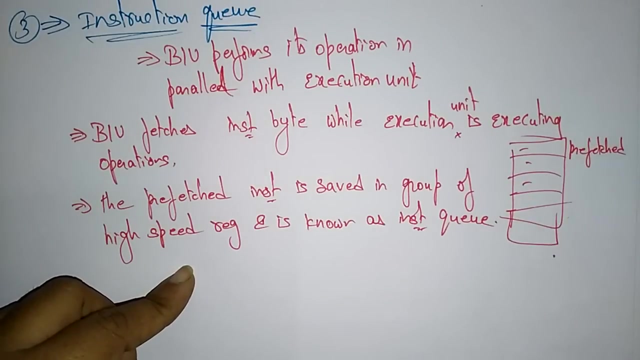 as instruction can. instruction queue is? is each sentence, every instruction distress. having this, two bites instruction will store. this is a pre extension instruction, That is, that has to be executed by the execution unit. that prefetched instructions is saved in a group of high speed registers. 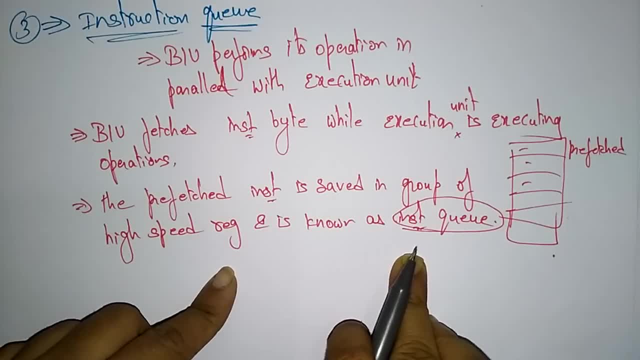 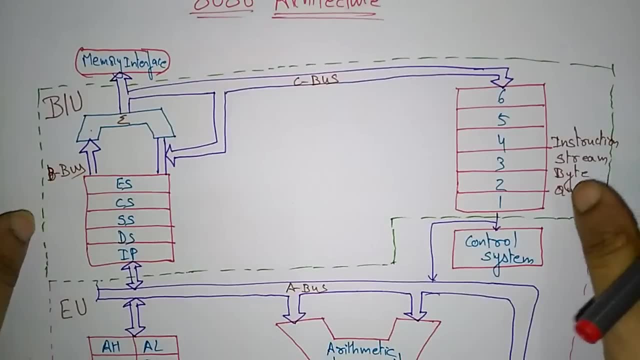 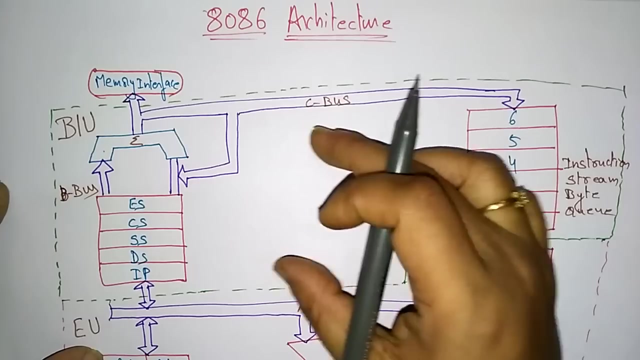 So this instruction queue is a high speed register that you have to be noted. Okay, that is saved in this instruction queue. So let me see. let us see the diagram: internal architecture. So this is 8086 architecture. So I said that 8086 architecture is divided into: 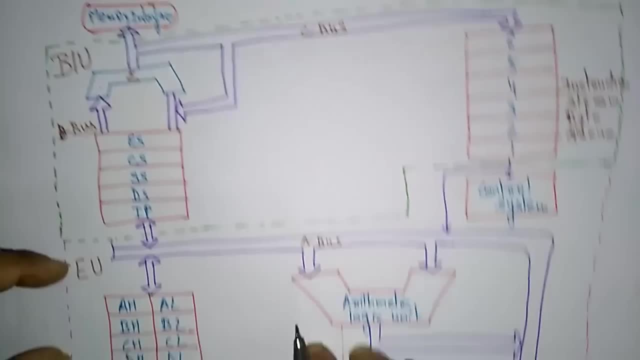 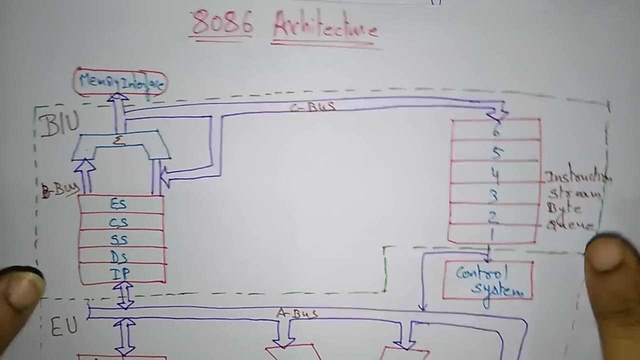 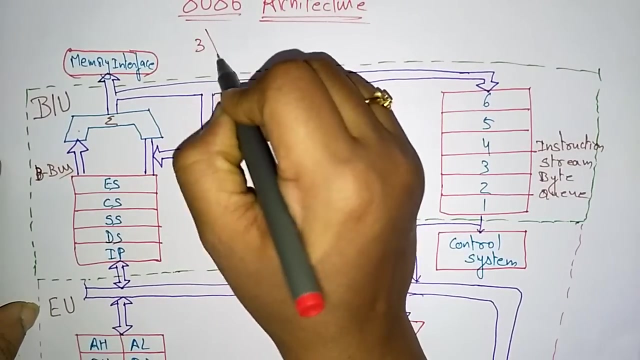 two units: One is a bus interface unit and next is the execution unit. So I already talked about the bus interface unit, So let me clear the functions that are. this bus interface unit will do So. I said the bus interface is divided into three functional parts. Okay, three functional.